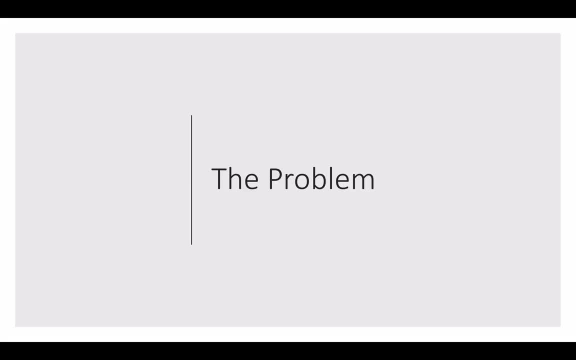 of the original object and copy their values to the new object. Nice, but there's a catch here. Not all objects can be copied this way. Some objects can have private fields which are not accessible from the outside, So you need to know exactly how many fields are there. 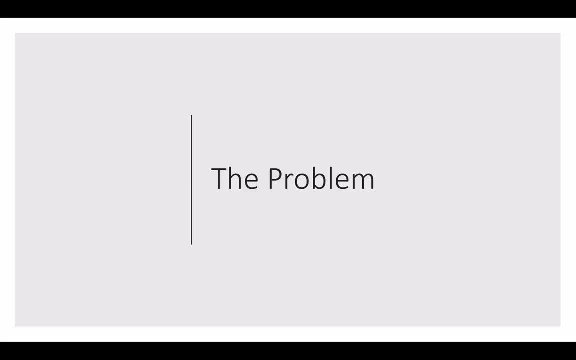 in the object, And your copying code will heavily depend on the number of fields and attributes you have in the classes, And you have to copy them one by one, by one. Also, since you don't have access to the private members of the class, you actually cannot copy those members. 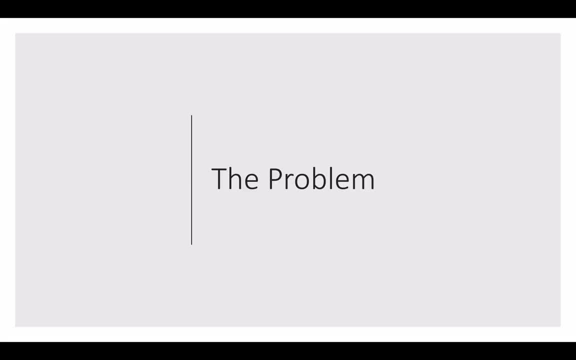 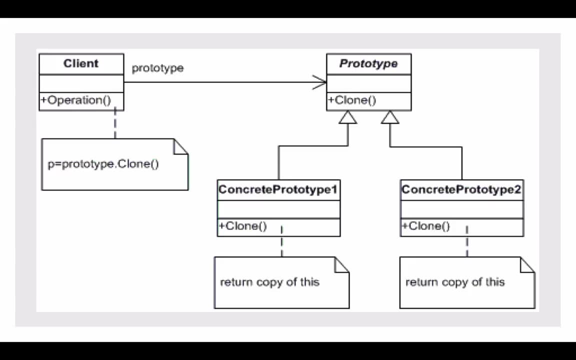 because you don't have access to them. So how does prototype pattern solve this problem? Let's have a look at the UML diagram. All right, so here's our UML diagram. The prototype pattern delegates the cloning process to the object themselves, which means: 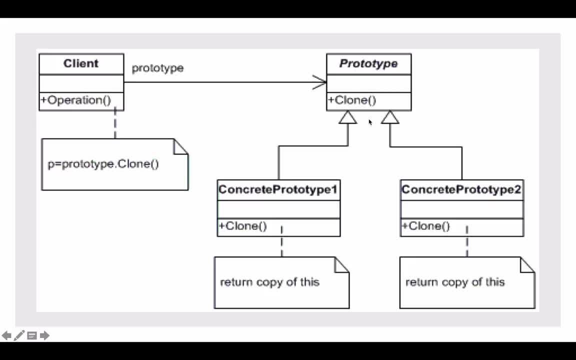 that it declares a common interface for all objects that allow cloning. It allows cloning objects without tight coupling to their classes. Usually, prototype interface contains a single clone method. So, as you can see, here we have the prototype interface, which exposes one clone method. 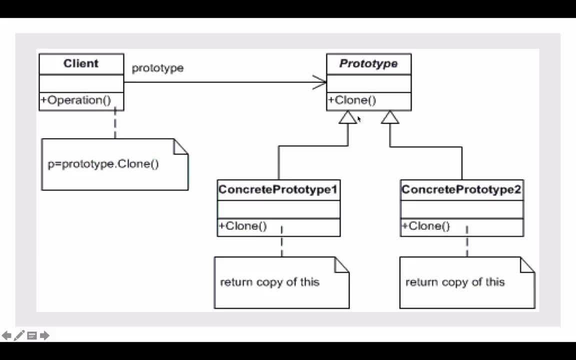 The implementation of this clone method is similar for all the classes. All these implementing classes need to do is to create a new instance of the same object and copy all the fields to the newer object and return the object. Objects which can be cloned with this method are called prototype. 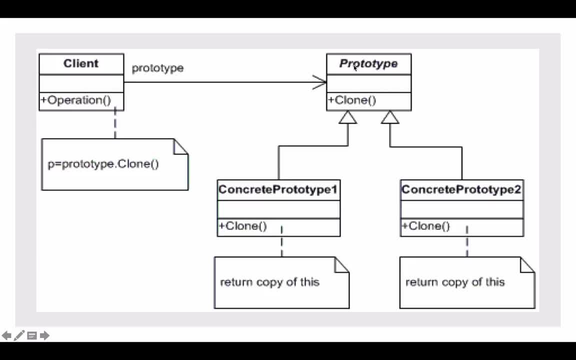 And especially when your prototype objects which have a very large number of fields, this method can be a better solution for copying the object instead of subclassing the object. All right, so let's look at how we can implement this in Java. All right, so let's take a look at the steps. 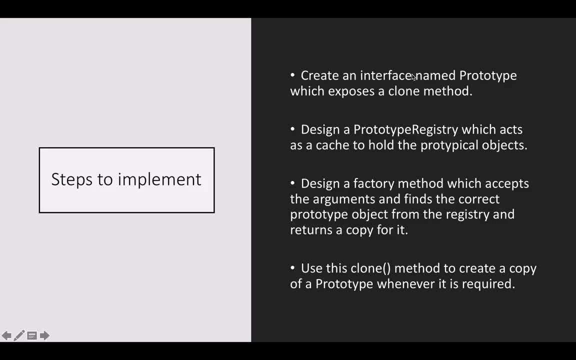 we need to implement. So the first step is create an interface named prototype, which exposes a clone method. OK, Then we'll be designing a prototype register which acts as a cache to hold the prototypical objects. Then we will design a factory method. 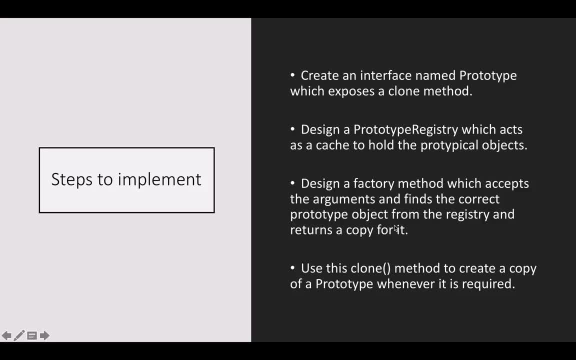 which accepts the arguments and find the correct prototype object from the prototype registry And whenever we will need a clone for that prototype object, we'll call the clone method on the prototype registry to get the prototype. So let's code this So here, as you can see, I have already. 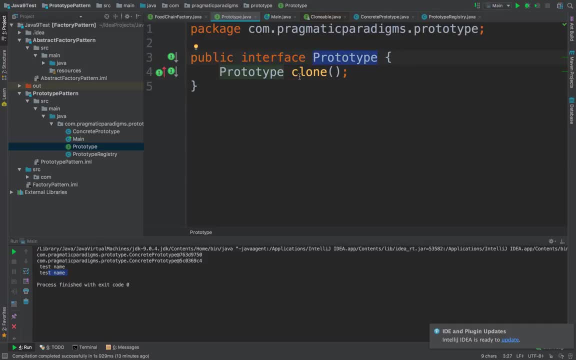 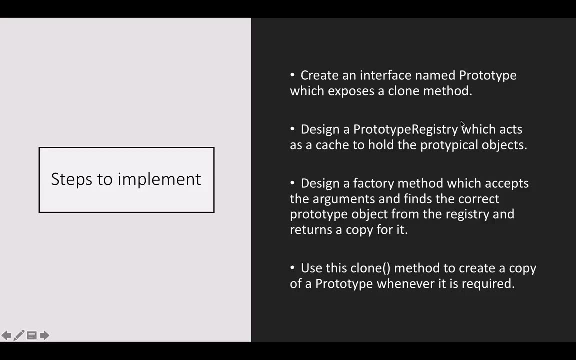 declared an interface called prototype, which has a clone method- OK- And which has a clone method which returns a prototype instance. The next thing we need to implement is a prototype registry which acts as a cache to hold the prototypical objects. 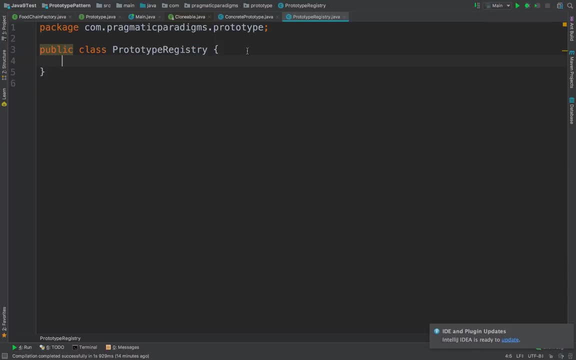 Let's go to the prototype registry. So this is our prototype registry class. Here we'll be implementing the cache which will hold the list of prototypes that can be cloned. So let's get started. First of all, we'll need a map, which 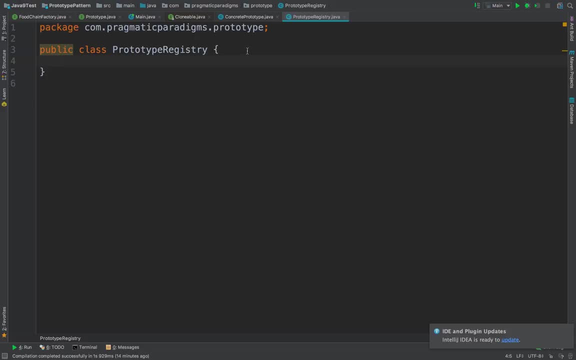 will hold a prototype key and a prototype value. So let's declare a map and let's quickly declare a constructor for this prototype registry which will instantiate this map. So here we are. Let's add the helper methods which will help us to run the map. 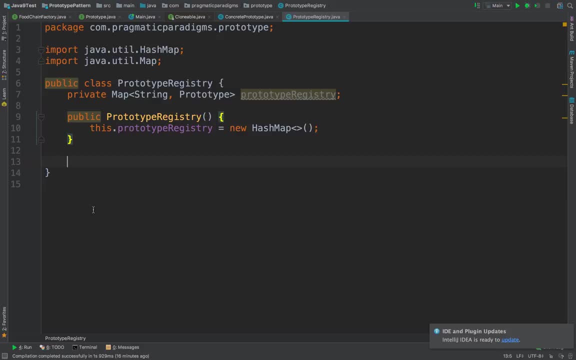 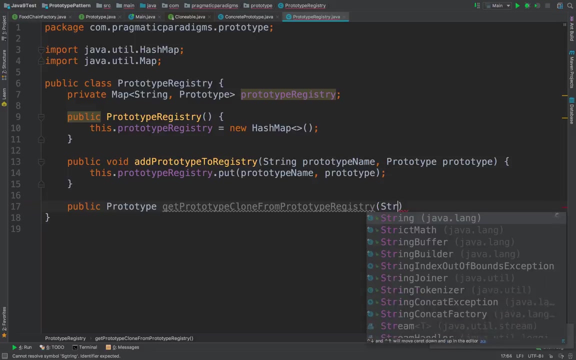 So here we are, OK, And this will help us to add prototypes to this prototype registry object and also add a method to retrieve the clone from the prototype registry. So here we have our prototype registry And we're going to call it prototype registry. 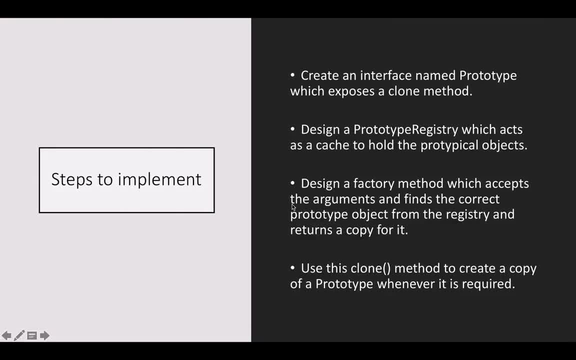 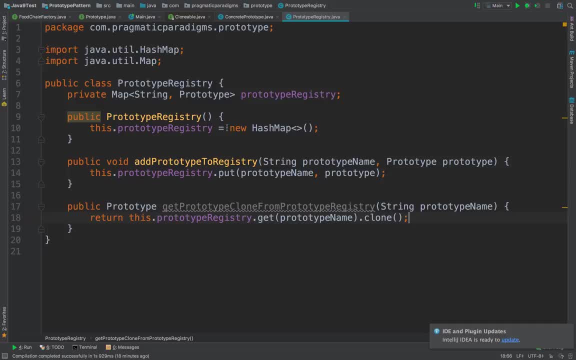 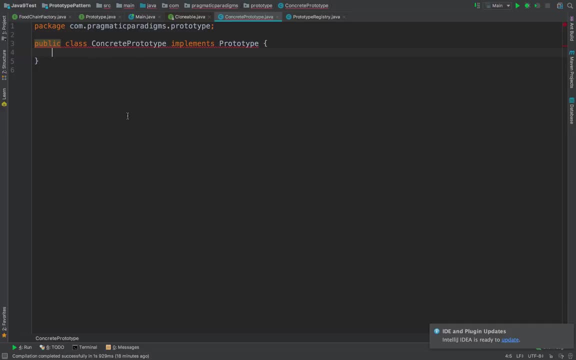 OK, So here we are. Our prototype registry class is ready. Let's go ahead and create an implementation for the concrete prototype, which will implement the prototype interface. So this is our concrete prototype class, where we will be implementing the behavior for the concrete prototype. 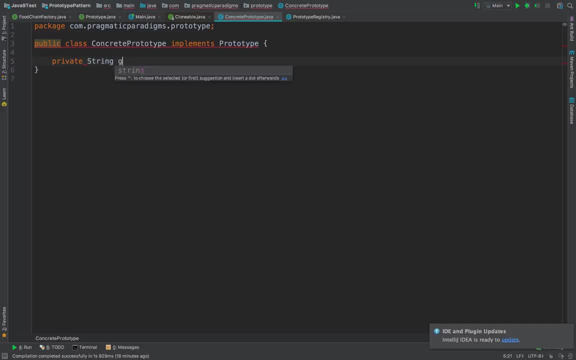 Let's quickly add a simple field called name-guid, And then let's add a constructor which will initialize this name. After that, we'll initialize one more constructor which will take the instance of this class. only just copy the contents of the object to the current one. 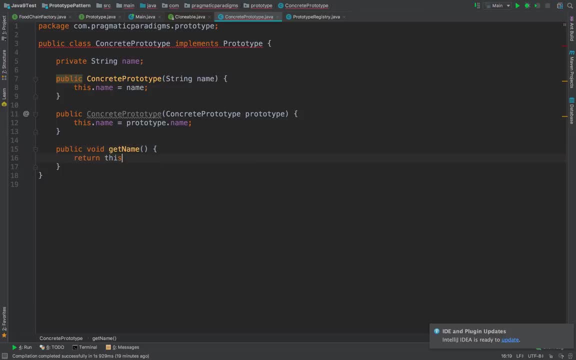 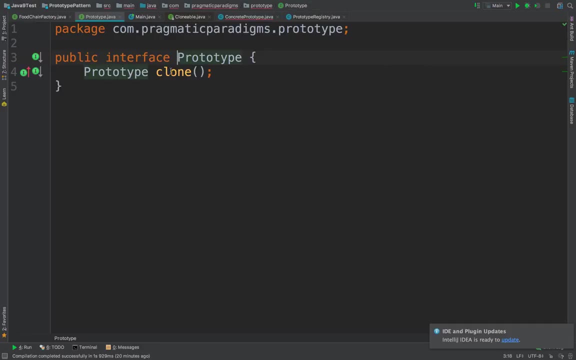 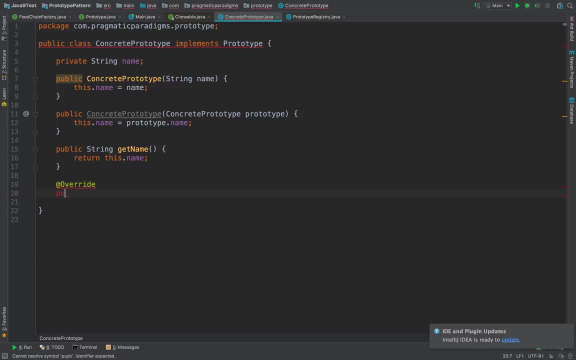 Also, let's add a method to get the name, And at the end we'll have to implement the clone method in this prototype. OK, So here we're going to create a new prototype interface which will override here, and this will return the concrete prototype. 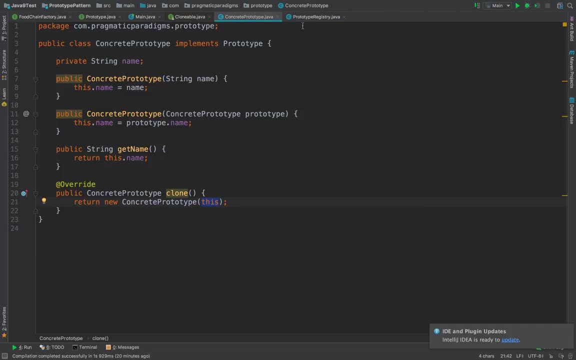 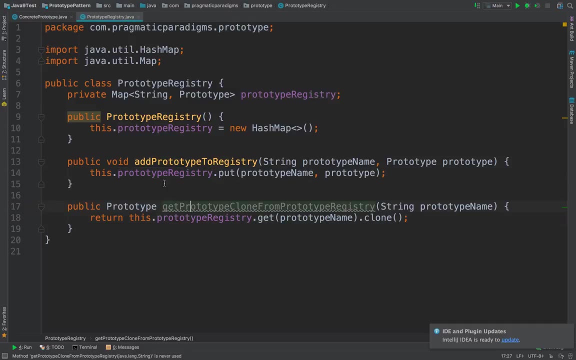 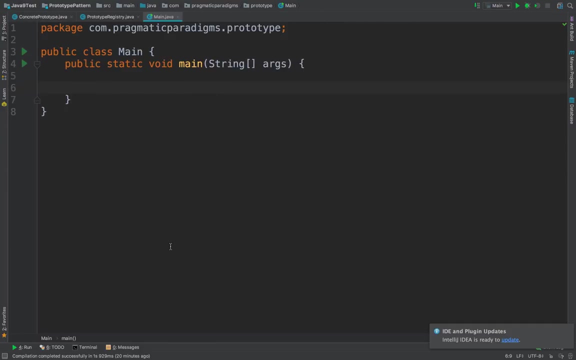 So we have designed all the classes which we need to execute this example. Let's quickly go ahead and add one more method, which will be the main method to execute the program. So what we'll do here is create an instance of the concrete prototype and we'll name it as the original. 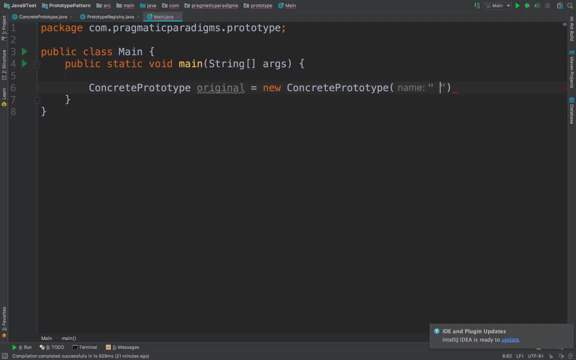 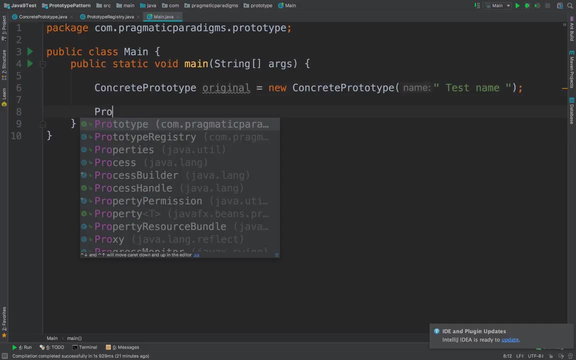 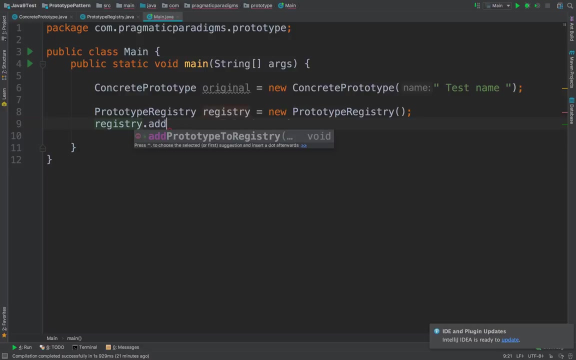 And we'll assign it the value of test name string. Then we'll create a prototype registry And register this prototype object which needs to be cloned. So we'll do registryadd prototype And we'll name it original And we'll pass the prototype value. 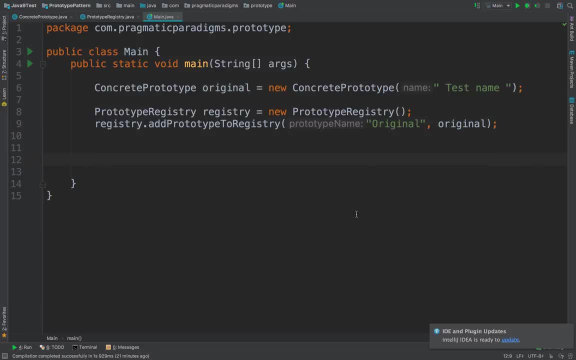 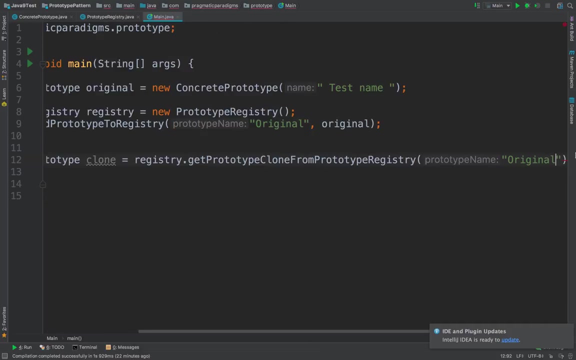 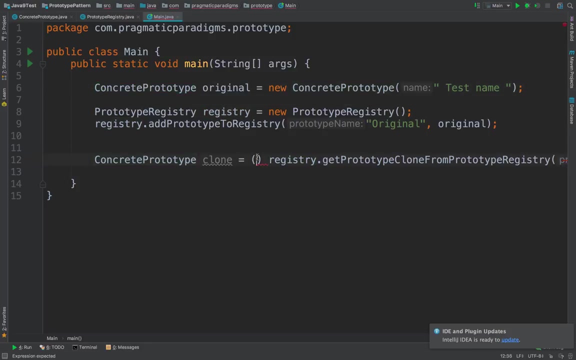 Now, let's say, after some time you need to clone this object. So Instead of instantiating, you can actually ask this registry object to provide you clone of the requested object, which is already there in the registry, And we can also typecast into the prototype we need. 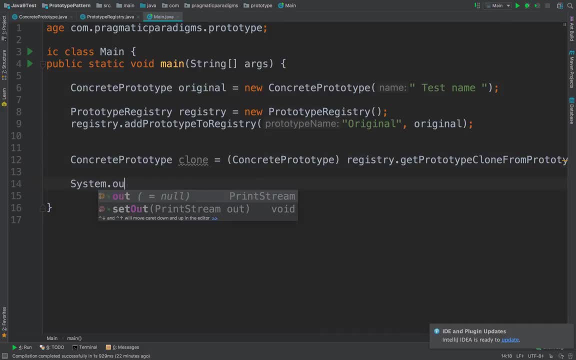 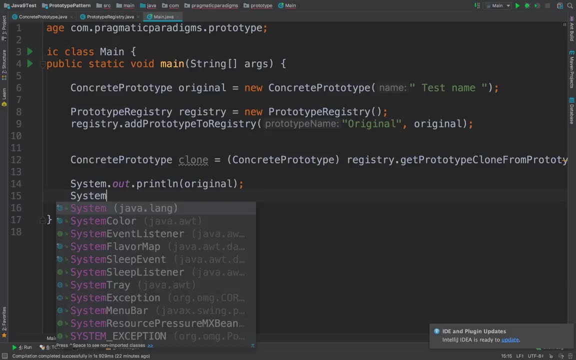 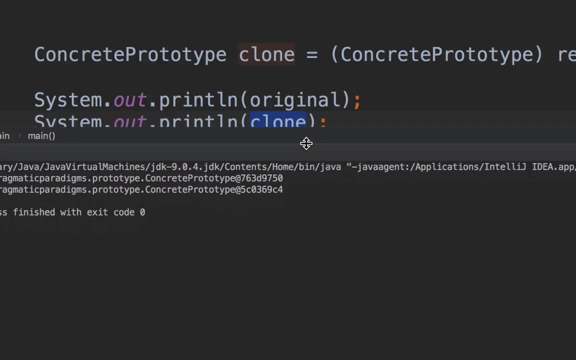 Let's try to print these two objects: First we'll print the original And then we'll print the clone. So after running this program, this original and this clone should have different objects. So as you can see here, this original and the clone.